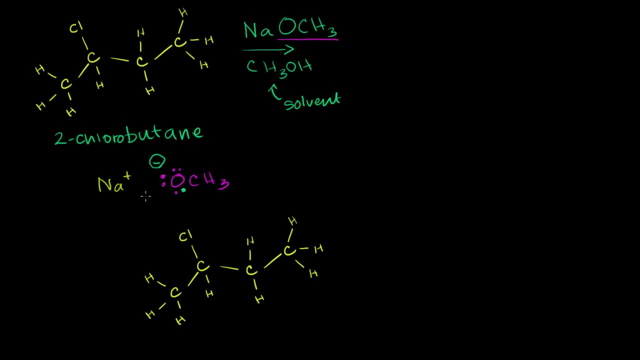 In solid form. when they're not dissolved, they form an ionic bond and they form a crystal-like structure. It's a salt, But when you dissolve it in something, in a solution- in this case we have methanol as the solution- they will. 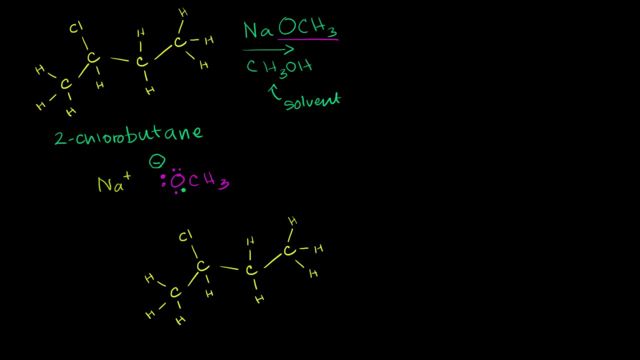 dissociate from each other. And what you have right here is this methoxide right here. This is a very, very solid. This is a very, very, very strong base. So this right here is a strong base And if you use the Lewis definition of a base, that 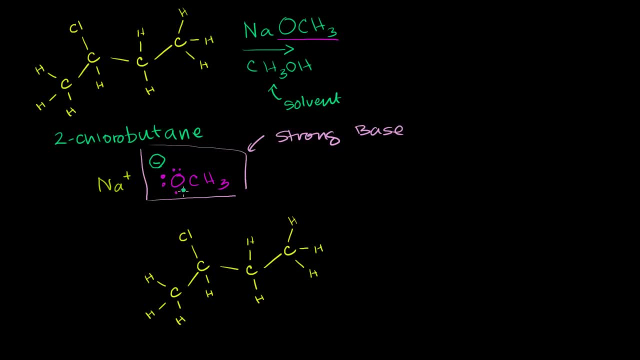 means it really, really, really wants to give away this nucleus to something. sorry, this electron to something else. If you use the Bronsted-Lowry definition, this means that it really, really, really wants to take a proton off of. 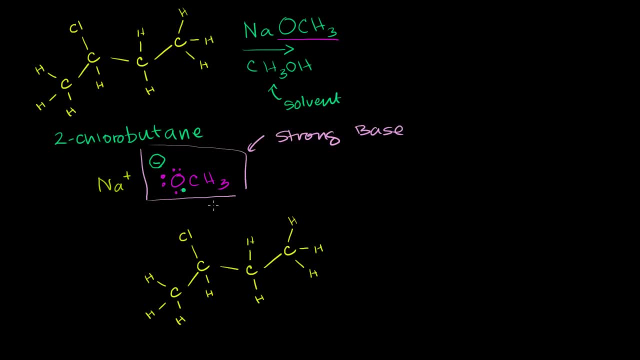 something else And in this situation, that is exactly what it will do, And I'll just give you one. I'll actually give you the most likely reaction to occur here, And we'll talk about other reactions and why this is the most likely reaction in future videos. 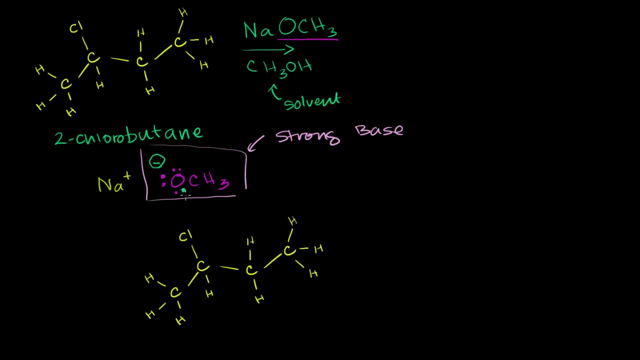 So it wants to nab a proton. It is a strong base. It wants to give away this electron. So let's say that it gives away this electron to this hydrogen right over here. Now. this hydrogen already had an electron. If it's getting an electron from the methoxide anion, the 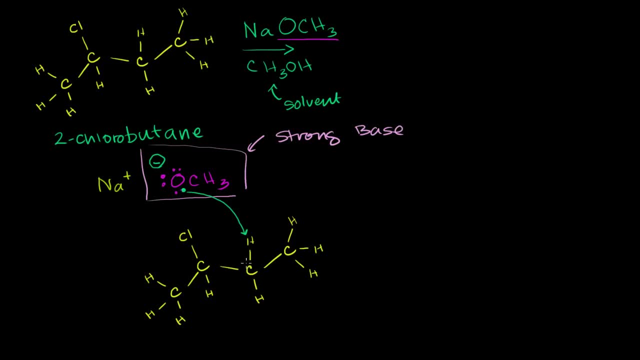 methoxide base, then it can give away its electron to the rest of the molecule. So now it can give away this electron to the rest of the molecule. Now carbon won't need the electron. Carbon doesn't want to have a negative charge. 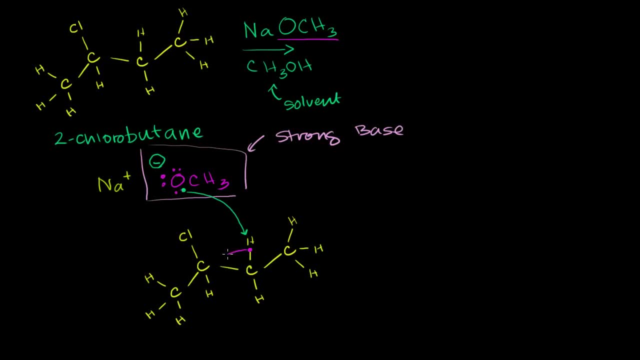 Maybe simultaneously. that electron goes to that carbon right over there, But once again this carbon doesn't want it. It only has four bonds, But what we see is we have this chloro here. This is a highly electronegative, I guess you. 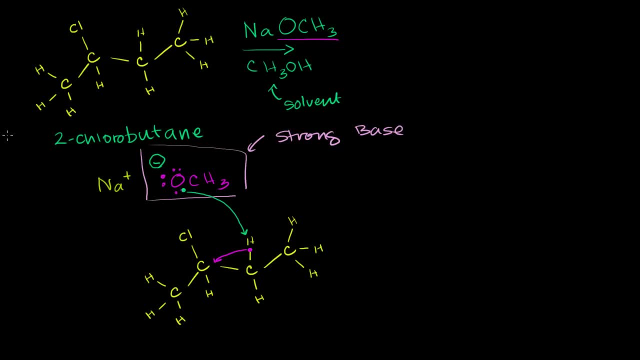 could call it a group. right now The chlorine is very electronegative, So the whole time the chlorine was already tugging on this electron right here. So now, all of a sudden, this is all happening simultaneously. When an electron becomes available to this carbon, then 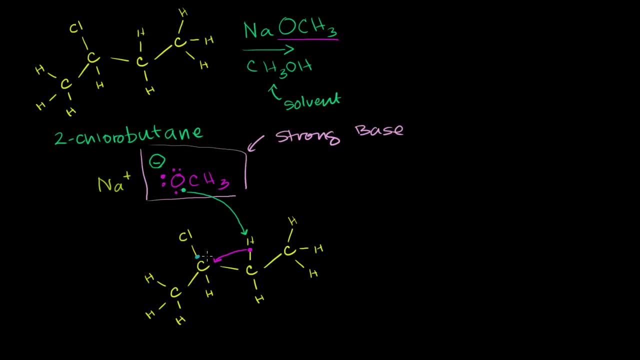 now this chlorine, this carbon doesn't need this electron anymore. the chlorine already wanted it. So now the chlorine can take it, It can take the electron And just like that, in exactly one step. let's think about what happened If all of this whole chain reaction- and I shouldn't call 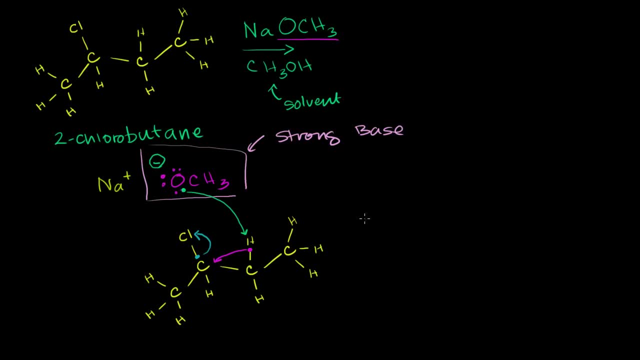 it a chain reaction. this simultaneous reaction occurred. what are we left with? So let me redraw my 2-chlorobutane, But I'm going to have to change it now. So now the chlorine. this has disappeared. So let me clear it. 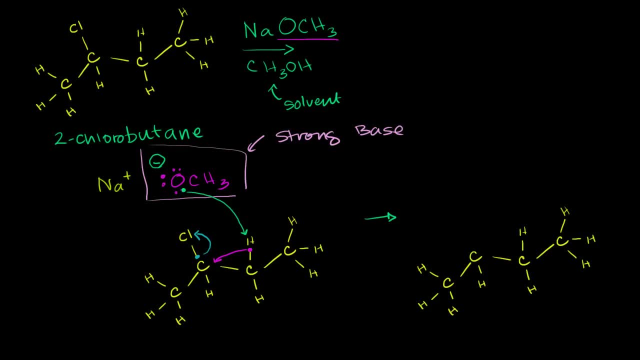 That's disappeared. The chlorine has now left. This chlorine is now up here. It is left. It had this electron right over there, which is right over there, And then the other, the electron it was paired with, that was forming a bond, is now also on the chlorine. 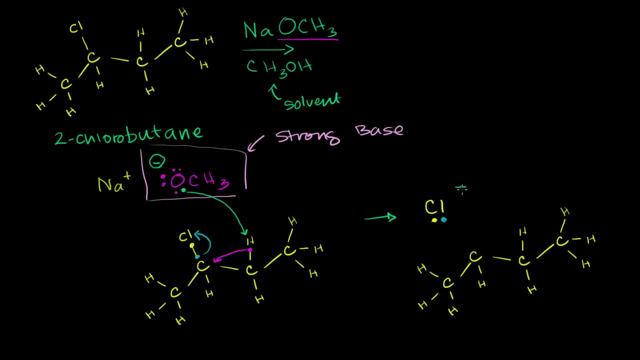 So now it becomes a chloride anion. So now it is a chloride anion. Let me draw the rest of the valence electrons 1,, 2,, 3,, 4,, 5,, 6.. And it had the seventh one right here. 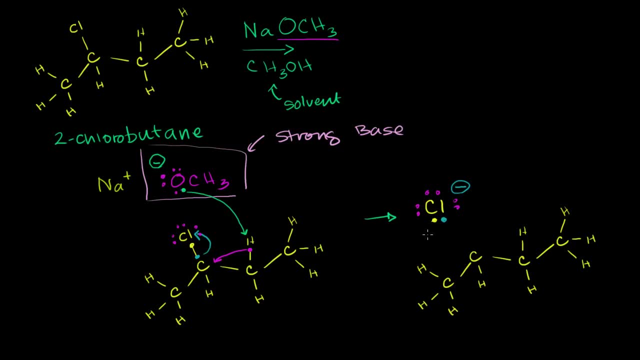 1,, 2,, 3,, 4,, 5,, 6.. 7,, 8 now. So it now has a negative charge. Now this electron up here. let me clear this part out as well. Now this electron right here, this magenta electron. 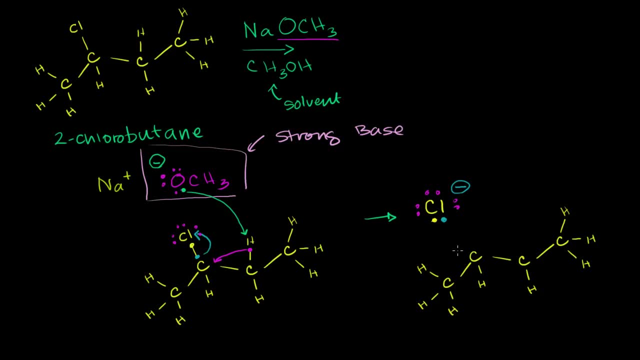 this is now given to this carbon. So let me draw it here, So that magenta electron is now given to that carbon. And if we look at the other end, The one that was paired with, that was bonded with it still is bonded with it. 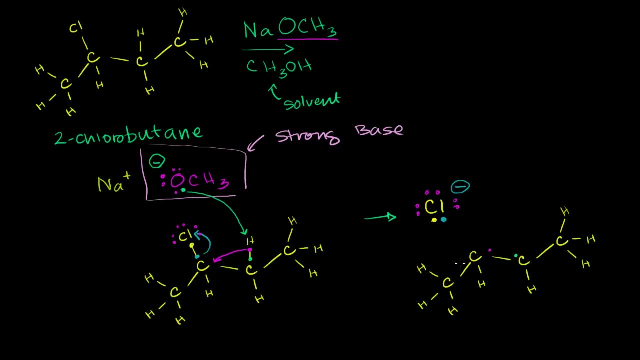 So that green electron is now still on that carbon. And now they are bonded, And now they're forming a double bond. So now they are forming a double bond. This all of a sudden has become an alkene, And now the methoxide took the hydrogen. 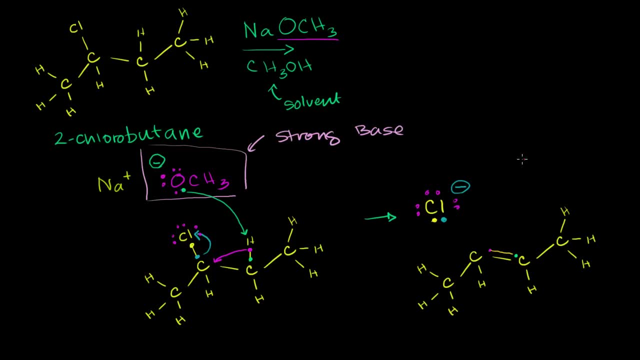 So let me redraw the methoxide, So OCH3.. The oxygen had 1,, 2,, 3,, 4.. 3,, 4,, 5.. It had 6, well, actually it had 8 valence electrons. 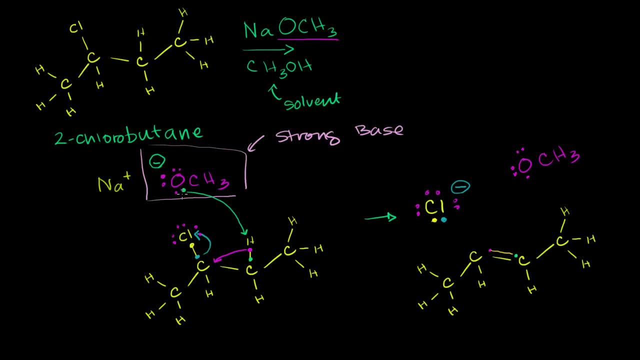 Actually it had 7 valence electrons, One with the carbon and then all of these 6 unpaired ones. Neutral oxygen has 6.. But now it gave one of them away to a hydrogen. It gave that green electron over there to the hydrogen. 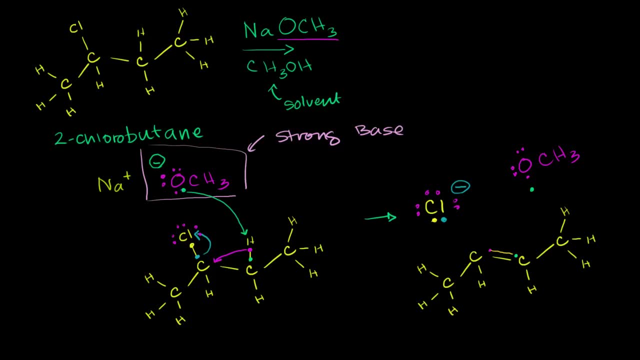 It gave that green electron over there to this hydrogen. Let me do it. I'll make this hydrogen the same color To this hydrogen right over here. so now this hydrogen, this hydrogen is now bonded with it. This hydrogen is now bonded with it. 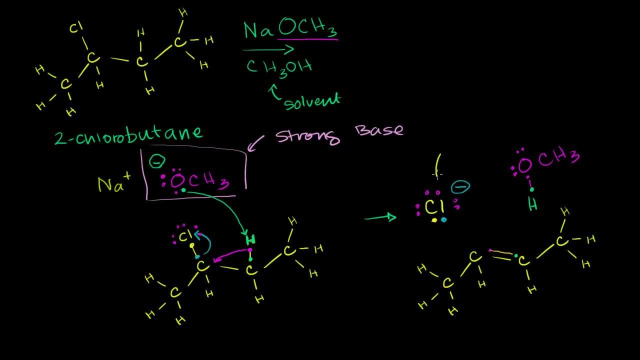 So what are we left with? We have a chloride anion, So this is chloride anion. We now have methanol. this was a strong base. now it has become it's conjugate acid, So now we have methanol. 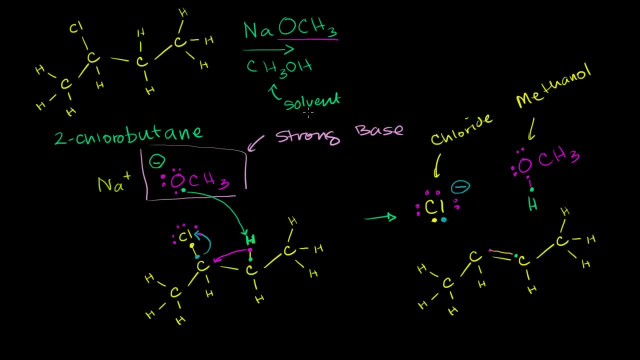 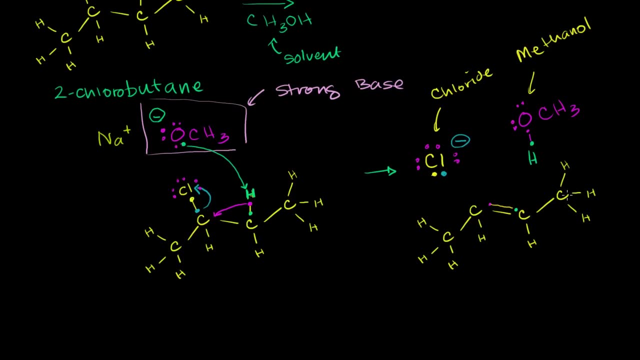 Which is the same as the solvent, Same as solution. So it kind of just- Or actually- same as a solvent. so it's now mixed in And now we're left off with 1,, 2,, 3,, 4,, still 4.. 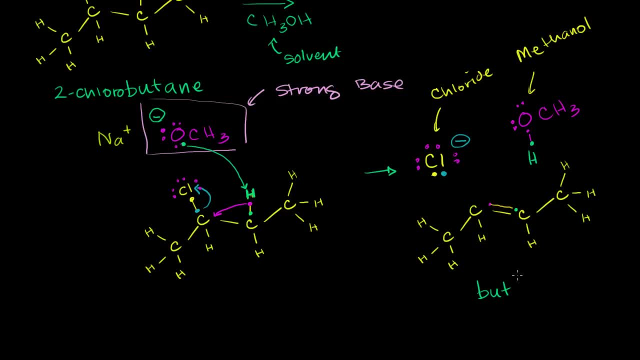 We still have 4 carbons, But now it's an alkene. We have a double bond, So we could call this but-2-ene or sometimes called 2-butene. So let's think about what happened here. It all happened simultaneously. 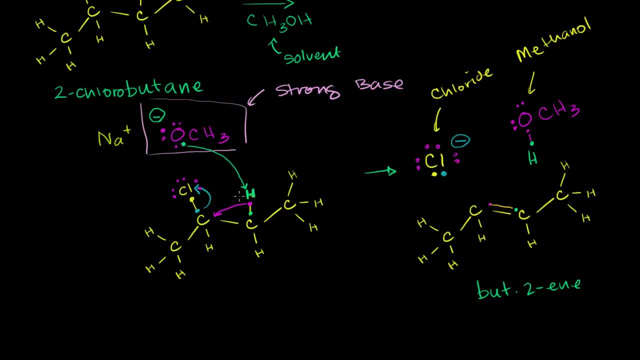 Both reactants were present. There was actually only one step, So this is the rate-determining step. So if we were to try to name it, we'd probably have a 2 in it someplace And something got eliminated- The chloride, or I guess you could call it the chloro group. 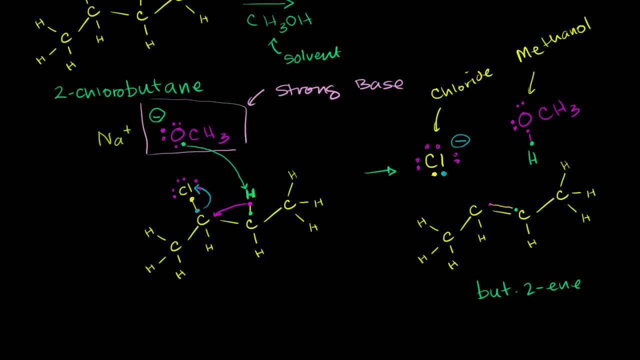 got eliminated. It left. It was a leaving group in this situation, So this was eliminated And this type of reaction where something is eliminated and both of the reactants are Participating in the rate-determining step, and we only had one step here, so that 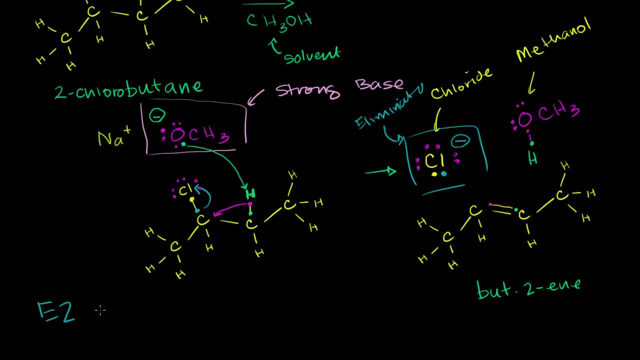 was the rate-determining step is called an E2 reaction And once again E stands for elimination And the 2 stands for that. both reactants involved in the rate-determining step. We had one reactant and two reactants.